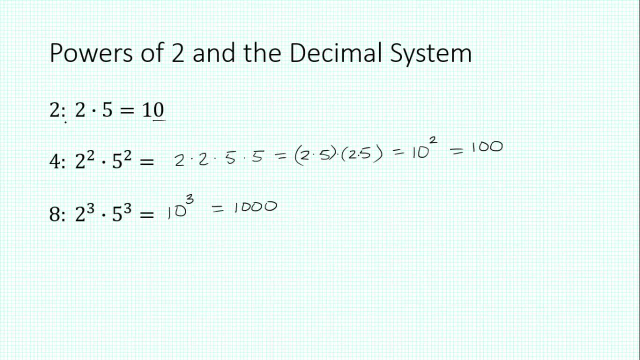 So now look at the pattern. 2 to the 1 is a factor of 10 to the 1,, which has one 0.. 2 squared is a factor of 10 squared, which has two 0s. 2 to the 3rd is a factor of 10 to the 3rd, which has three 0s. 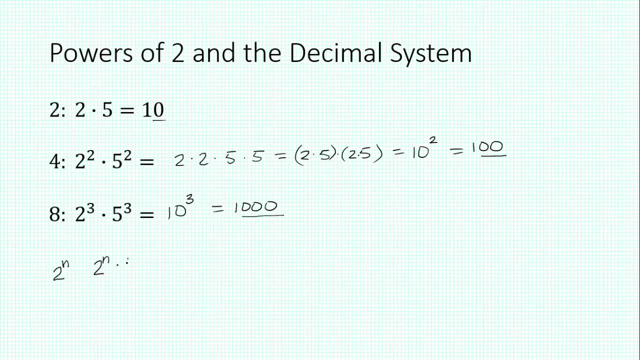 So we could extend this 2 to the n times 5 to the n, which is the same as 10 to the n, which will look like 1, followed by n 0s. All of this background is why the rule for powers of 2 and divisibility works. 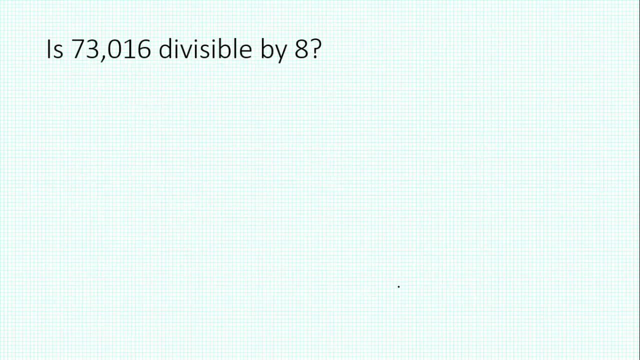 Let's see more. Here's an example: 73,016.. Is it divisible by 8?? Well, keep in mind that 8. is 2 to the 3rd, So we know that 10 to the 3rd, or 1,000, is divisible by 8.. 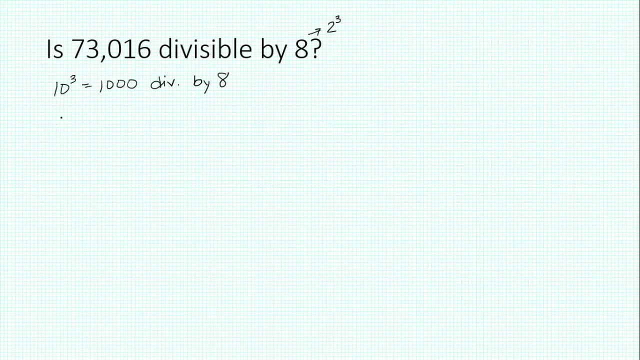 So let's rewrite 73,016 as a multiple of 1,000 plus 16.. Automatically this is divisible by 8, because 1,000 is divisible by 8. When you multiply it by 73,, you get another multiple of 8,, and 16 is also divisible by 8.. 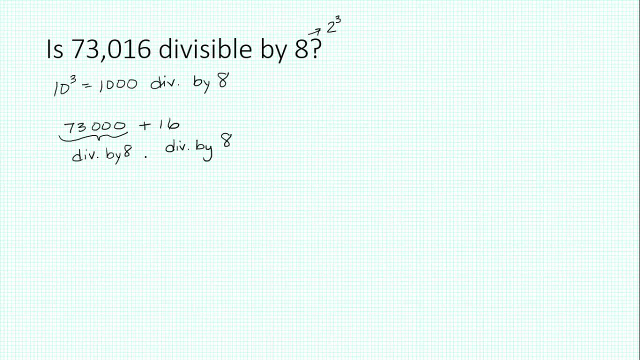 We have a sum of 2 numbers that are both divisible by 8. A multiple of 8 plus a multiple of 8 creates another multiple of 8.. So the answer to this question is yes, And we're getting very close to using the rule. 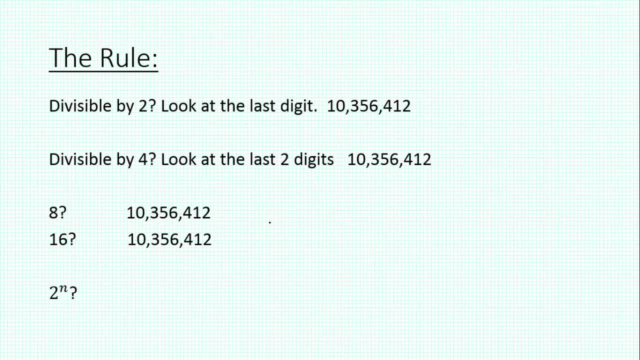 Let's see what it is According to our powers of 2 and powers of 10,. if you want to know if a number is divisible by 2, you just look at the last digit. The rest of it is a multiple of 10, which is a multiple of 2.. 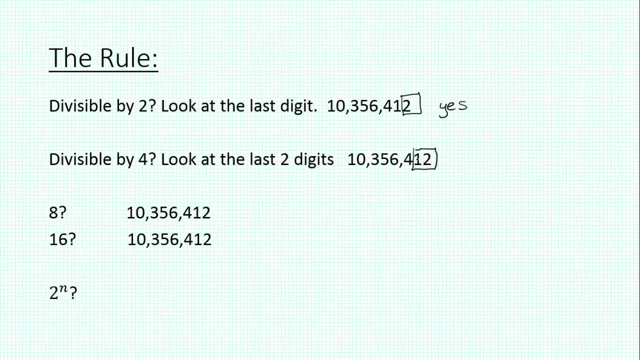 For 4.. For 4, you only need to look at the last two digits, because the rest of it is a multiple of 100. That's a multiple of 4.. For 8, it starts to get a little more challenging to work out in your head. 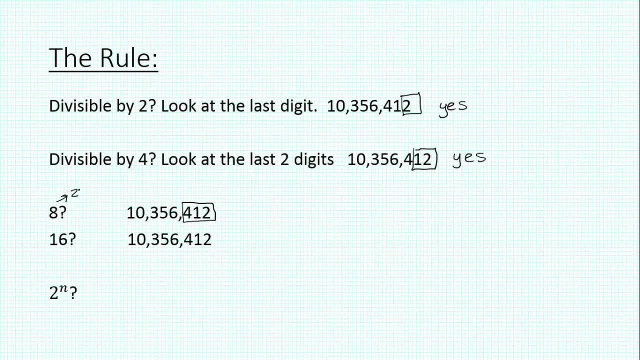 But you should focus on the last three digits, because 8 is 2 to the third And for 16,, since it's 2 to the fourth, you're going to look at the last four digits. It turns out that 412 is not divisible by 8..